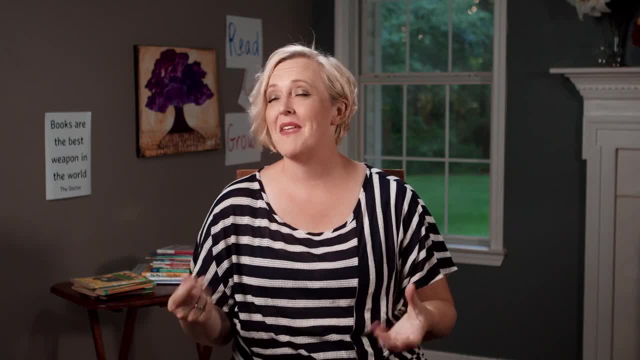 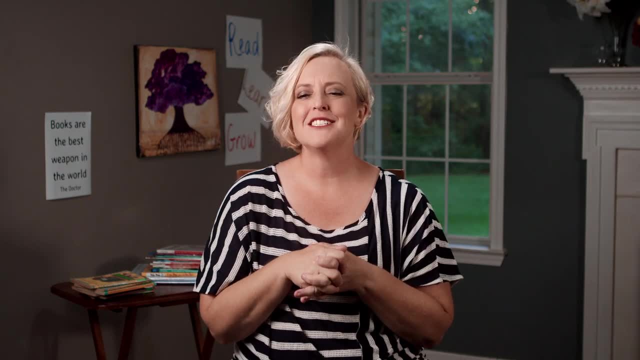 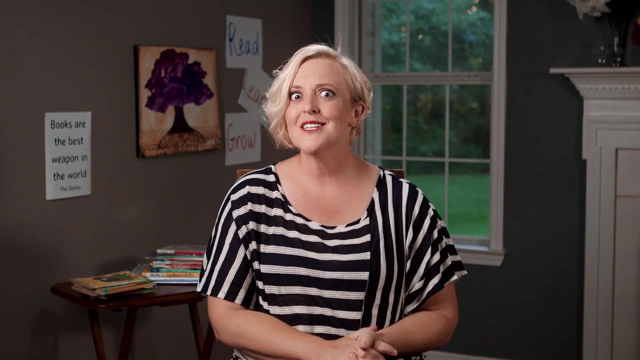 I like it when I meet new people and invariably the sort of conversation ends up in education seems to naturally happen with me And they'll ask: oh so you're homeschooling? I'm like yes, And then I'll often say: and I actually unschool. And it's really interesting to see the sort of the 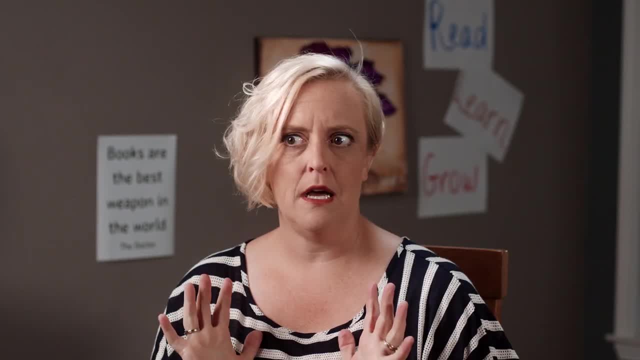 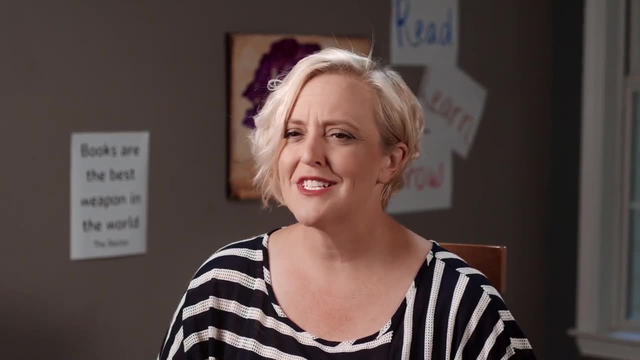 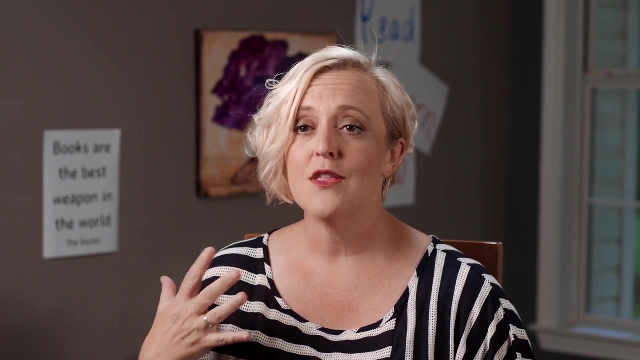 reactions that you get from people. You get that whole- I don't know what that is look. or you get the oh, you're one of those, are you Sort of looks. And I love unpacking, unschooling for people. I really do, because I just truly enjoy it, And I think the more that 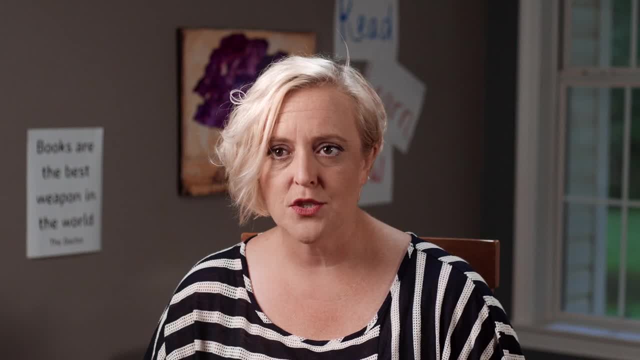 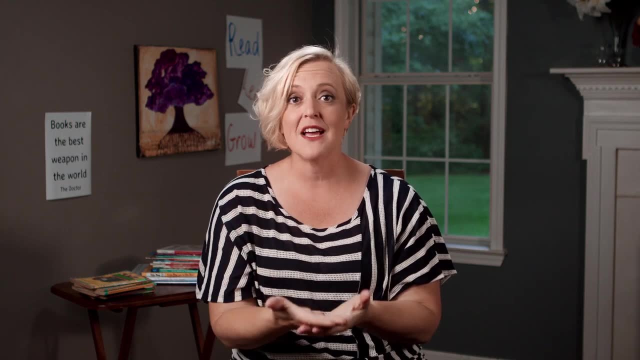 people realize what it is and as a way to homeschool. it's a beautiful thing, And so this is why I love bringing some of these videos, And I've done this. We've been talking a bit about unschooling, and we looked at how to unschool math and how to unschool science. 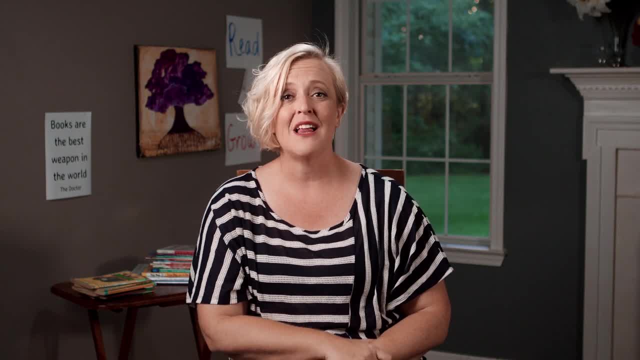 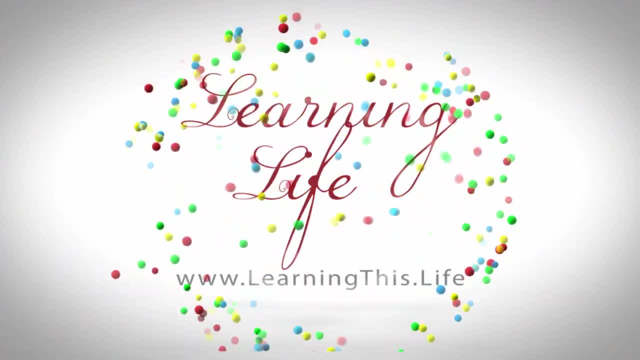 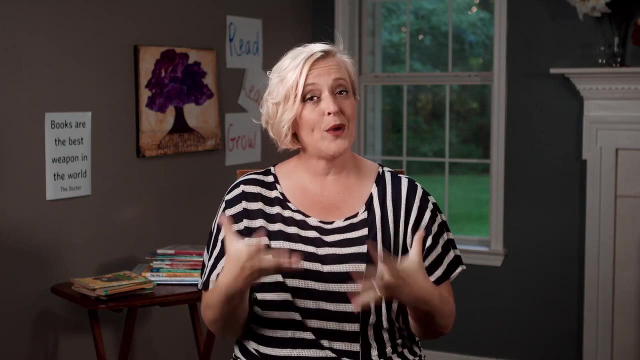 Today I want to look at how to unschool language arts. Hi and welcome to Learning Life And thank you for joining me today as we unpack unschooling language arts, because you know, when you're an unschooler, so often you get the 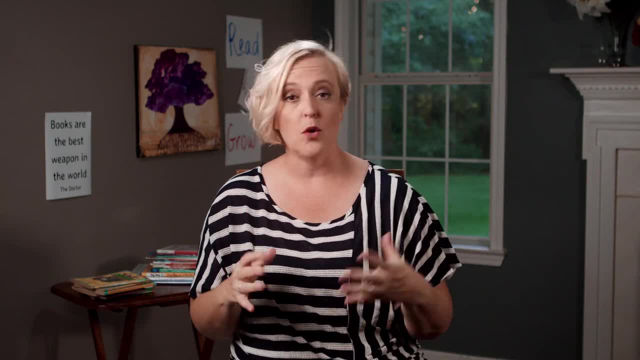 question: well, how do you like, how do you, how do you do this, How do you? and then the whys. but you get the question: well, how do you like, how do you, how do you do this? And then the whys. 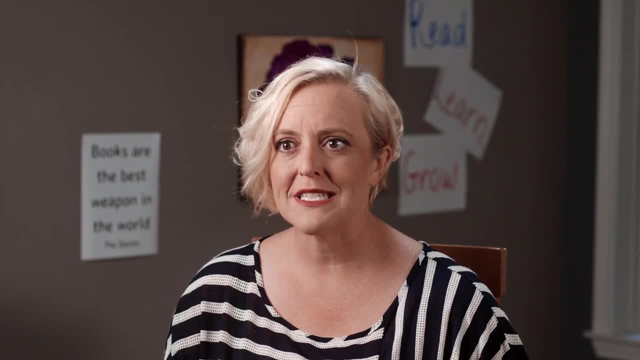 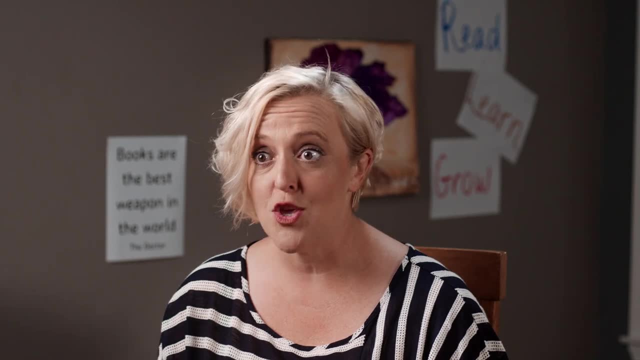 usually it's the how do you like? how do you unschool math? You know, and I said we covered that. You know, when we have questions, it's always great to go and find answers, And maybe you've been wondering how to unschool language arts and you ended up here today. Well, thank you. 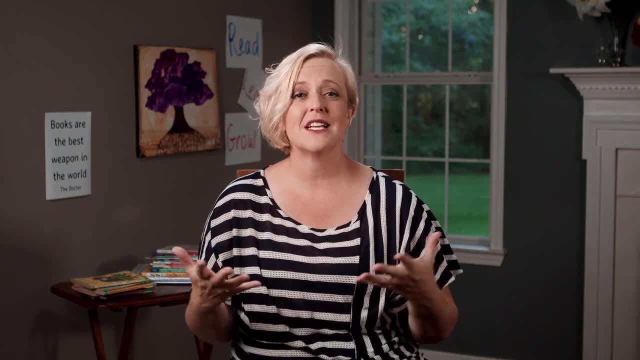 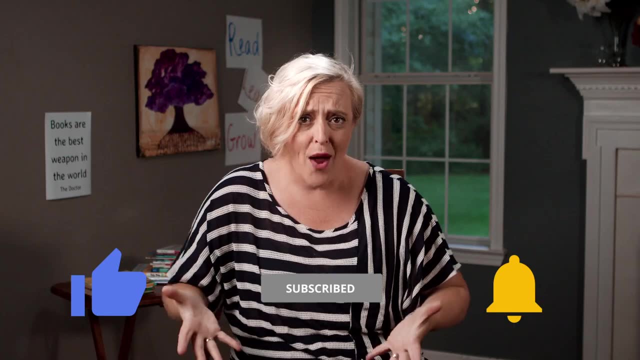 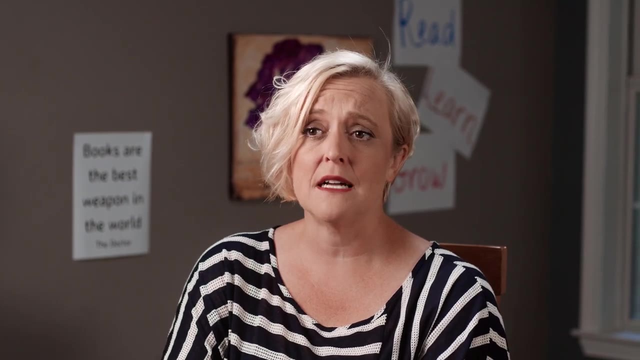 and welcome, And for those that have been joining me on this journey, you know what? thank you for being part of this community. Hey, like, subscribe. tell your friends you know what is language arts? Hey, I get that a bit. You know, when I started a teacher's college, that was when, like the whole, 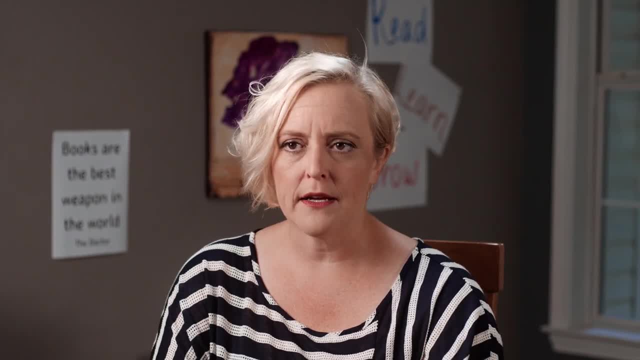 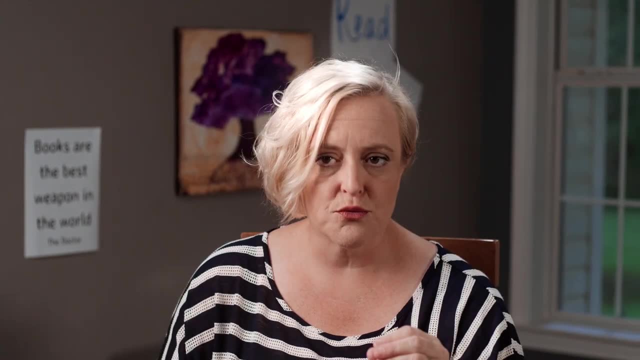 shift from just English or, you know, reading, writing became like language arts And really it's just. it's a curriculum that involves the language skills. It's not just reading, It's not just writing. We're putting it together And you know, there's just all the different methods that. 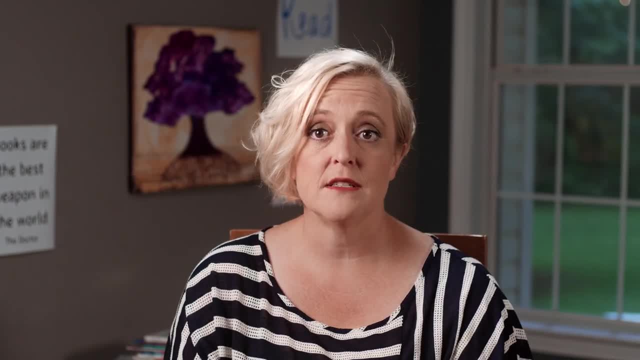 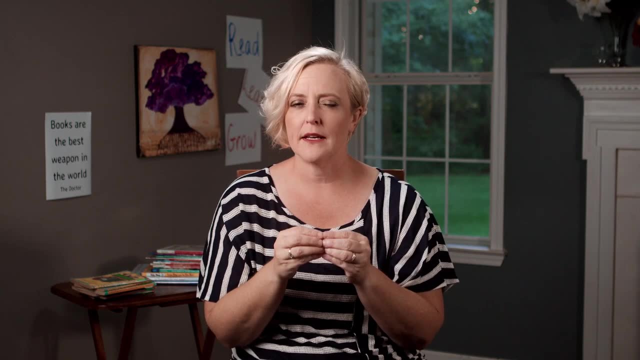 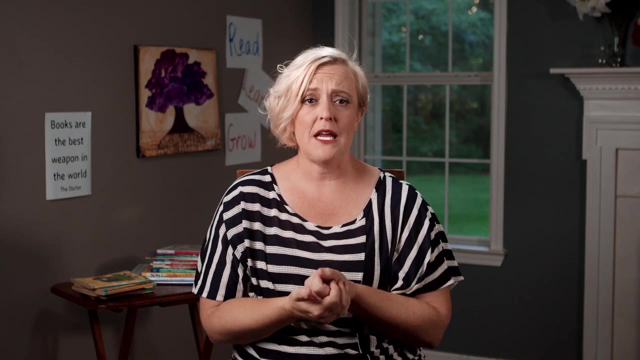 we can be using language in written and spoken form. That's what it is, But really we break it down mostly to reading and writing. So, as I'm talking about unschooling language arts, it's really unschooling like that: reading and writing. You know there are so many ways like to learn it. 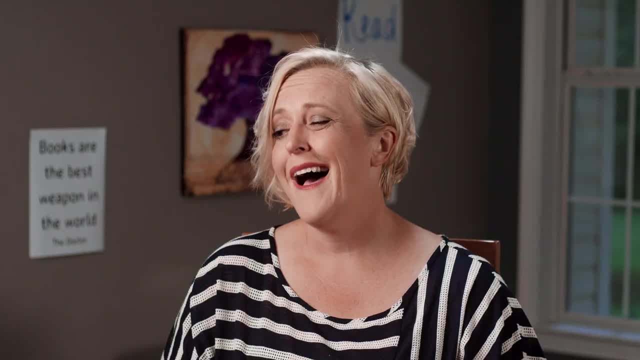 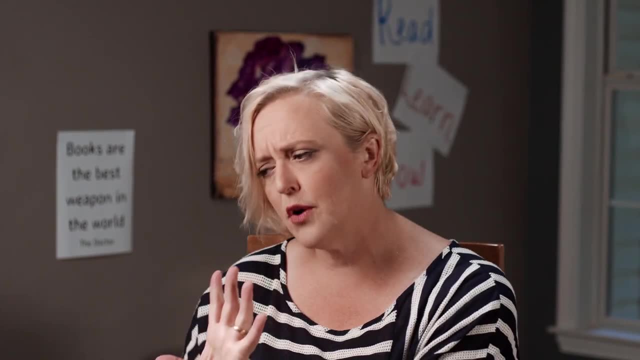 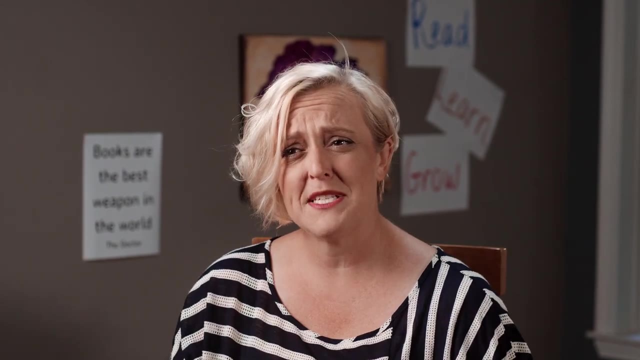 and there are so many curriculums out there that do it. But what I don't like is when it seems to just break up. you know, we've got our spelling and our grammar and our vocab and it's this, and I'm like, oh, it's a way that I don't like to teach. You know. I'm like, why are we separating? 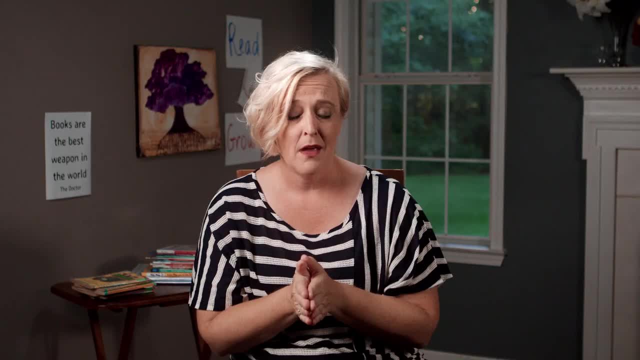 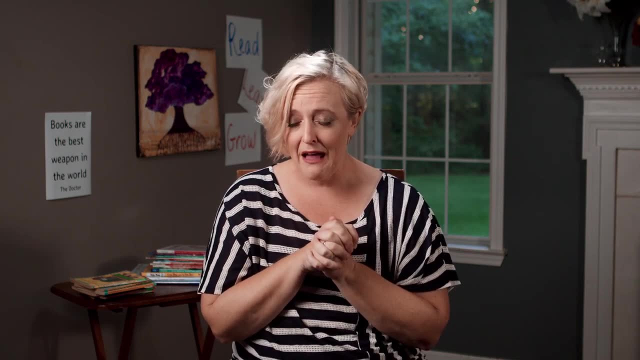 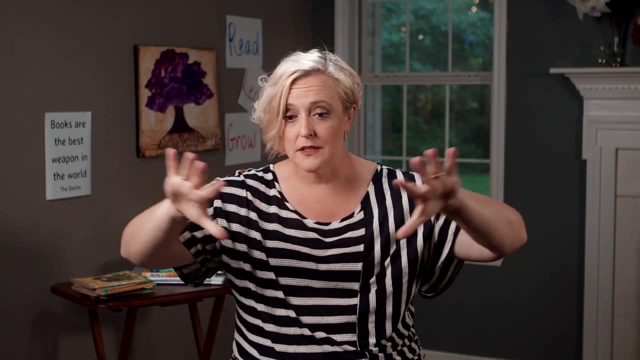 all of these things And they really, really belong together. And oh, you know, when I started teaching sixth grade here, my first year of teaching, I had to learn how to diagram sentences in order to be able to teach it. And I remember, like at this interschool, like teachers conference, asking: ah, why do we do? 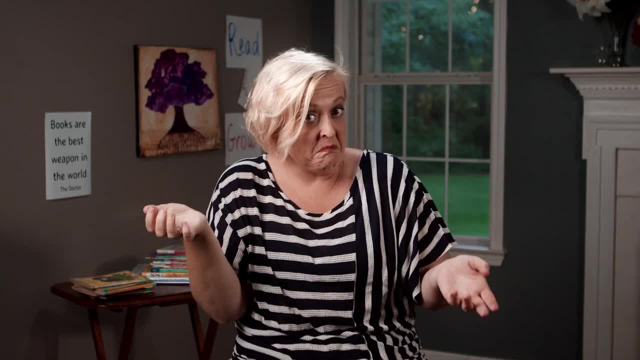 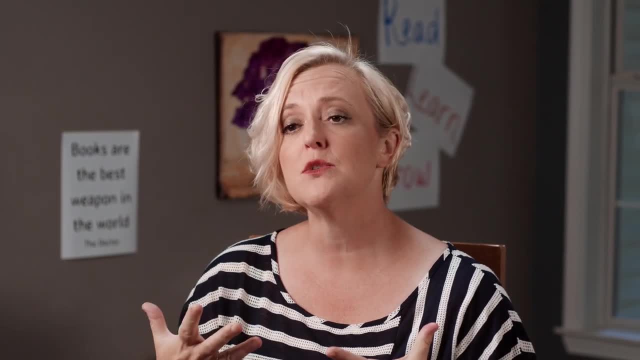 this And most people were like I don't know. I think there was one person who's like: well, it makes you a better writer, And I'm like: does it? Does it Like how? I mean, these were genuine questions, um, because I still struggle with diagramming sentences and 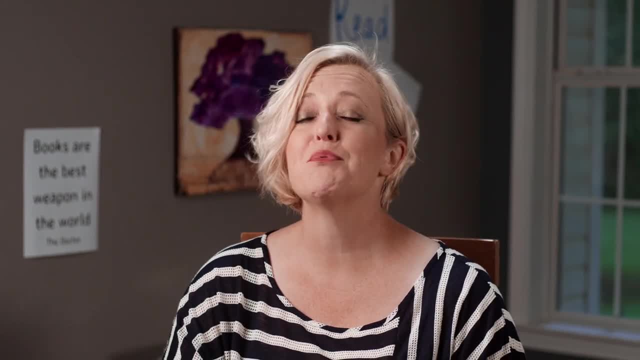 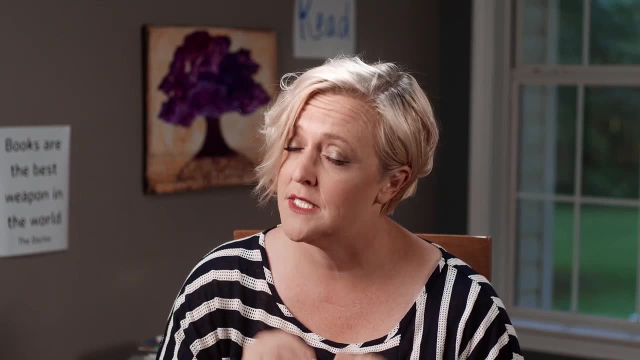 the reason why. but you know what? I also struggled being able to pronounce interrogative, because I still naturally want to say interrogative, because you interrogate someone in an interrogation. but I digress, Let's get back to unschooling language arts. 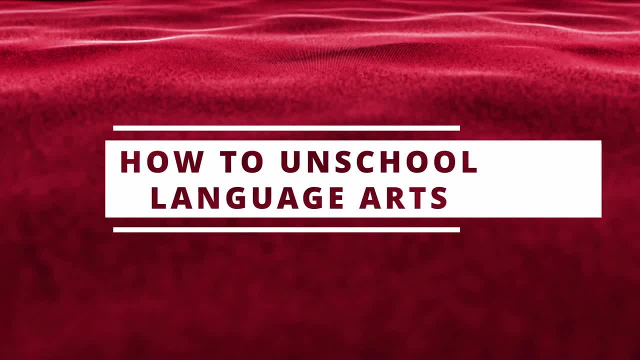 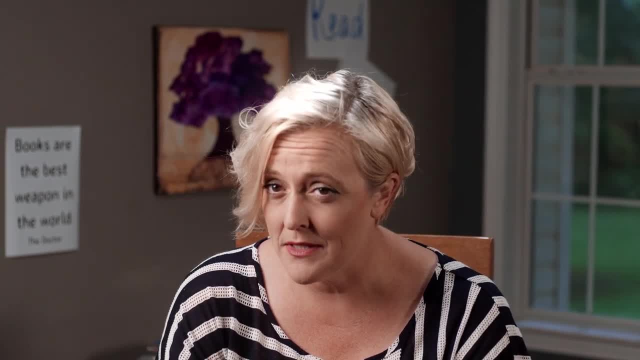 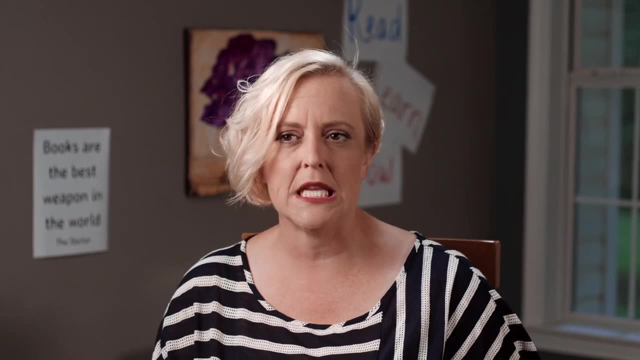 How do you unschool language arts? Wow, Are you ready? Let's have a language rich environment. And you're asking: hmm, what does that mean? It means that we have access to books and to written things and things that we can write, that we are communicating. Okay, We are using language. 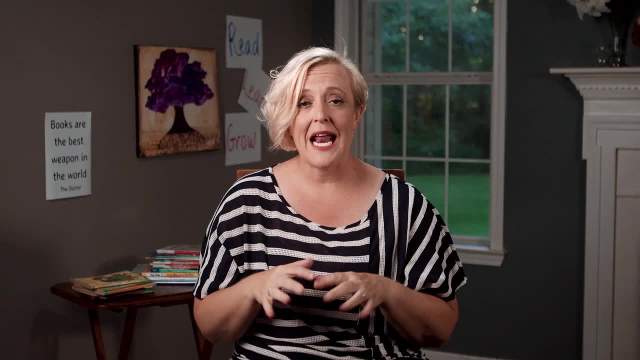 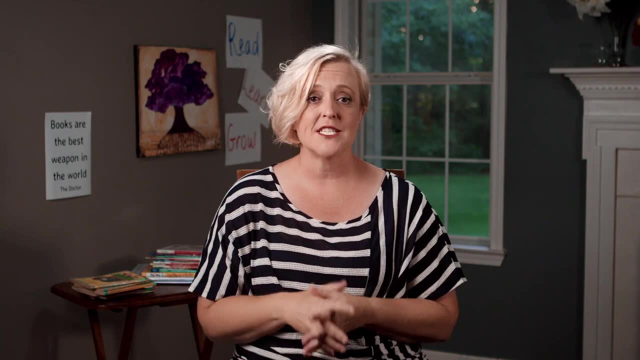 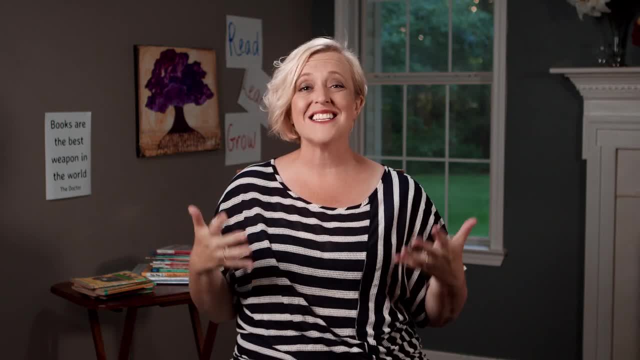 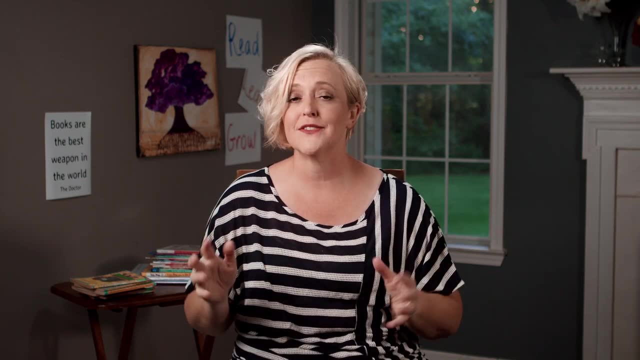 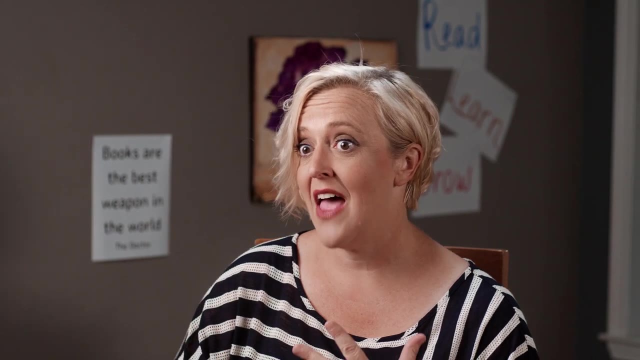 a book desert And we have lots of books We are reading aloud as a family. Okay, These are really great ways of doing it as a family. It's a great way to introduce many different styles of literature And, of course, both fiction and nonfiction, And in that and then from that, 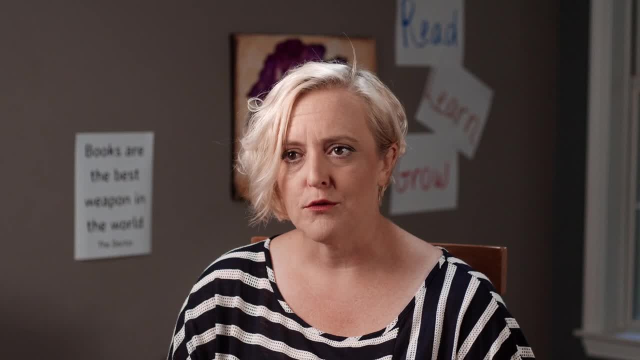 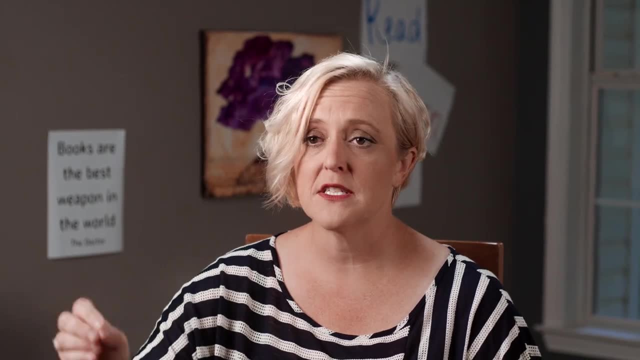 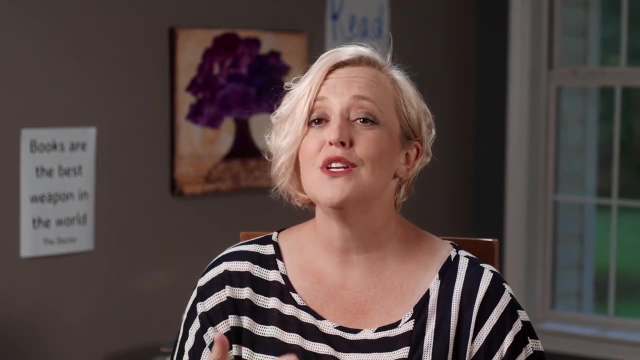 like we are modeling, reading and writing for our children. They need to see us do it, not just for work and not just for the things that we have to do to to keep the household running, but for enjoyment and for reaching out to somebody. Okay, We need. 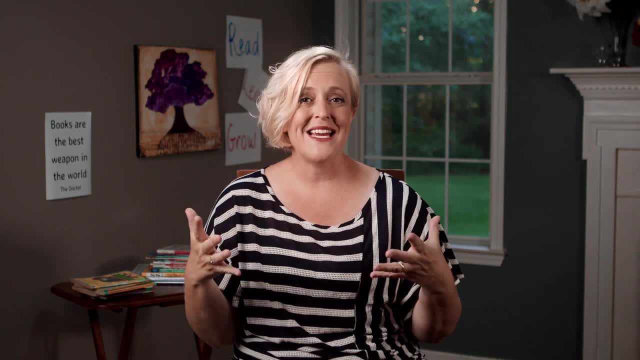 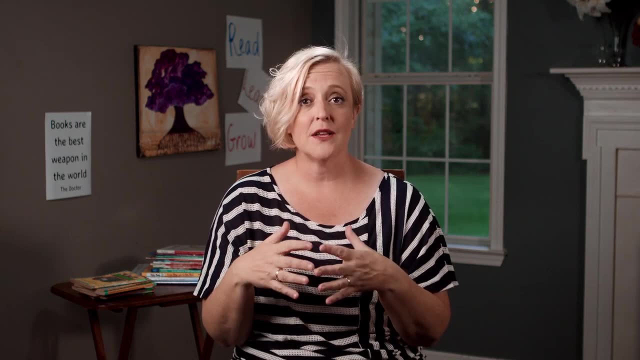 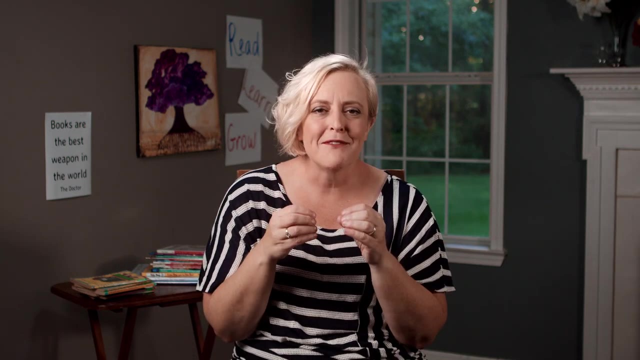 to model that for them And that's a great thing, you know, and it's including, like even I was telling my husband, one of my daughters has now started reading the way that I do. I use a lot of inflection. I use different voices for characters. you know, I'll bring my voice. 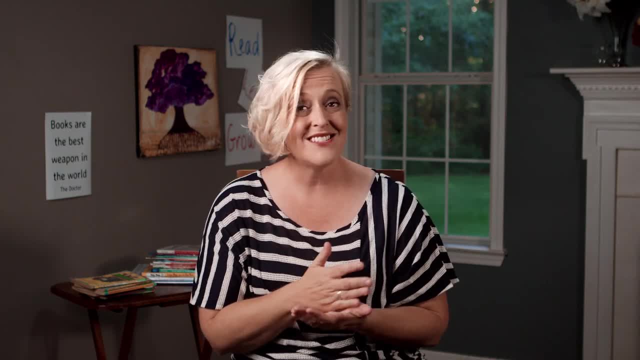 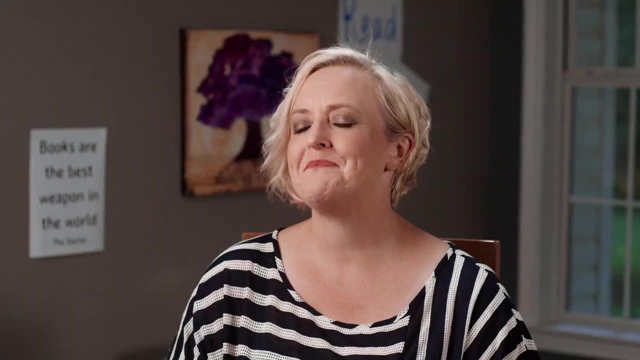 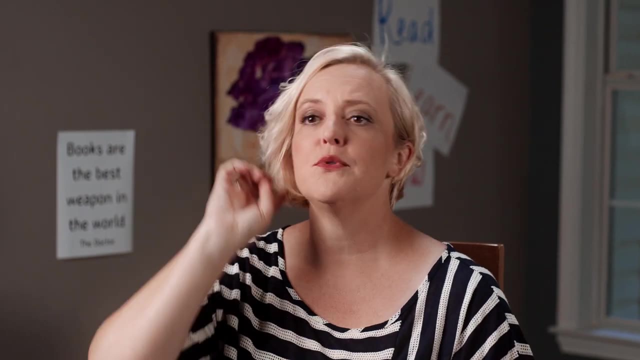 down And she, through me, modeling that. that's how she reads now And I love it. She's seven and she's already getting this reading expression happening. We do want to introduce phonics at a young age, but not through a curriculum. We want to do it. 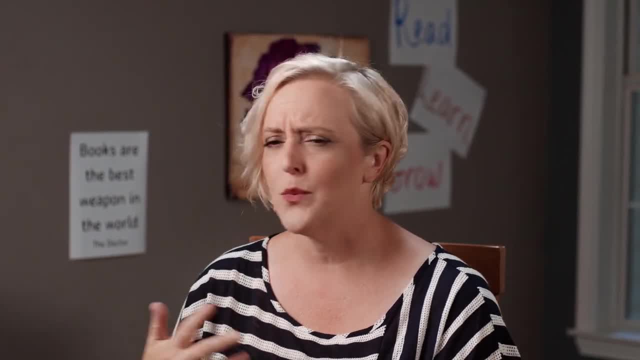 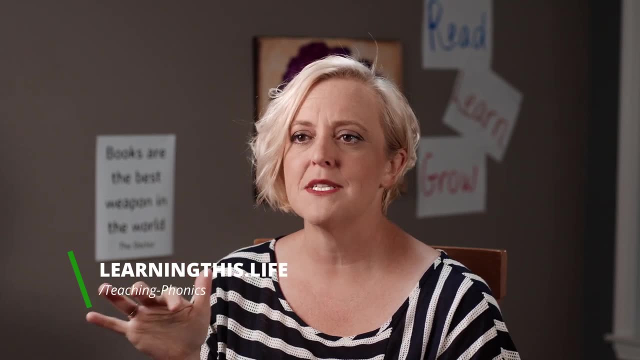 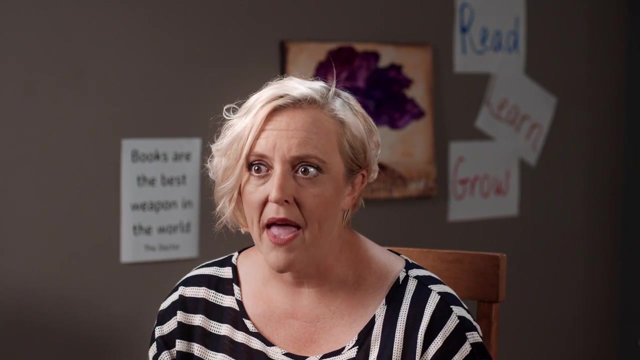 through games, And there are so many great and easy ways that we can introduce phonics to young children. In fact, go to my website, learningthislife, and I'll have some simple and easy ways that you can introduce phonics at a young age without it being anything you know major. 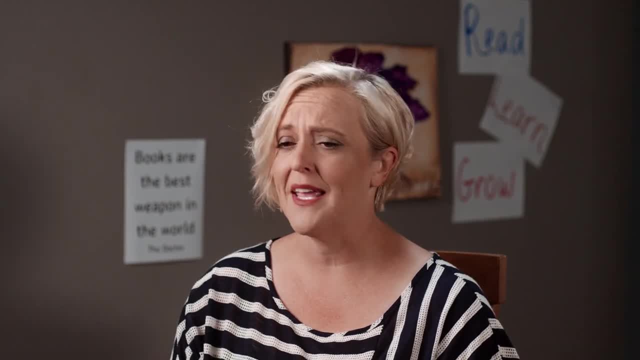 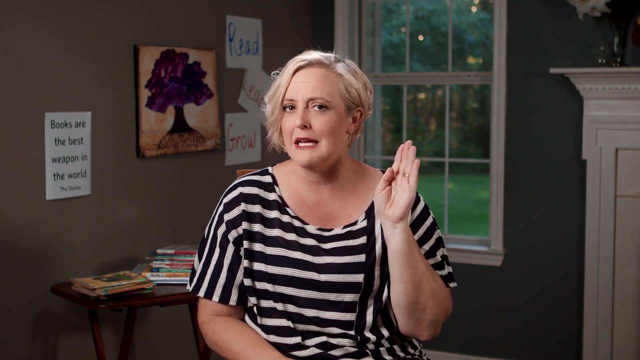 It's just something, it's fun And my girls still enjoy doing it. We want imaginative play. You know, of course, like have you ever listened to your children with the imaginative play And you realize that they're mimicking, like you and the things that you say or things that they've heard and you 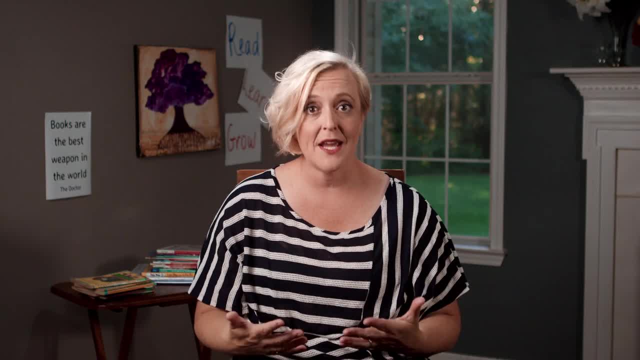 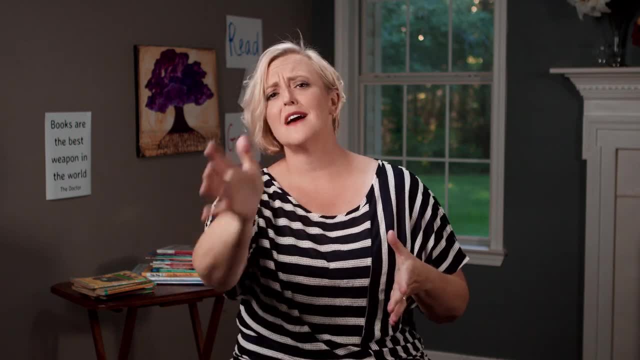 watch how their language develops through it and communicating meaning just through play. And so, yes, we work on our verbal communication and you know, we discuss things. We discuss what we're reading, We discuss what we're writing, We are engaged. 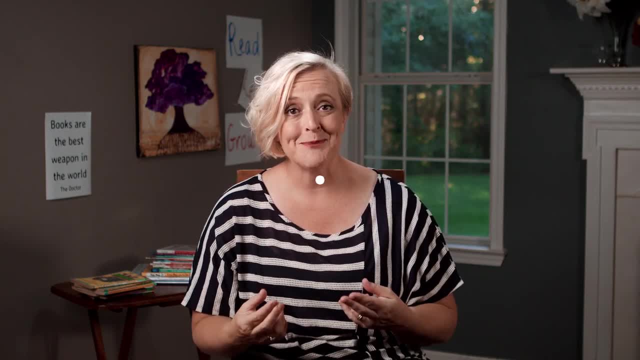 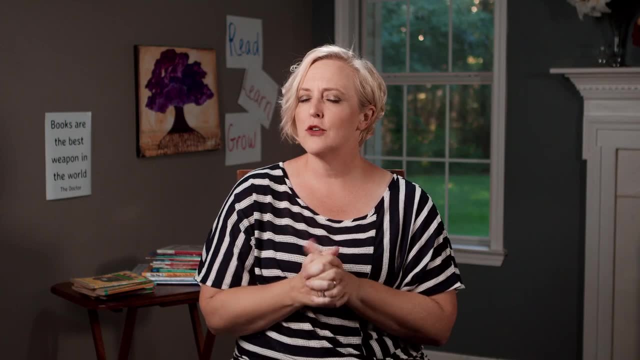 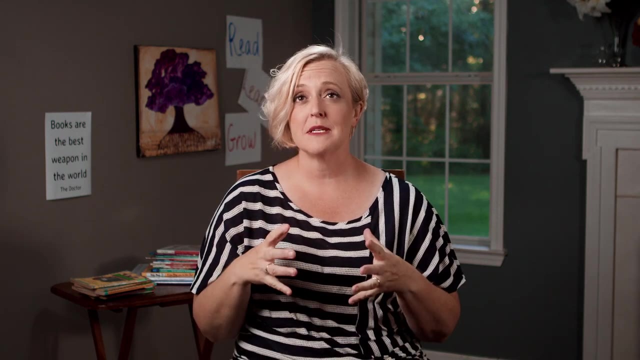 We are engaged in the written word and also in the spoken word. Activities for unschooling language arts. Can we learn grammar and spelling separately? Yes, Yes, we can, But we don't have to. okay, And I get some people are sometimes really worried. but if I don't learn it like this and I break it down, 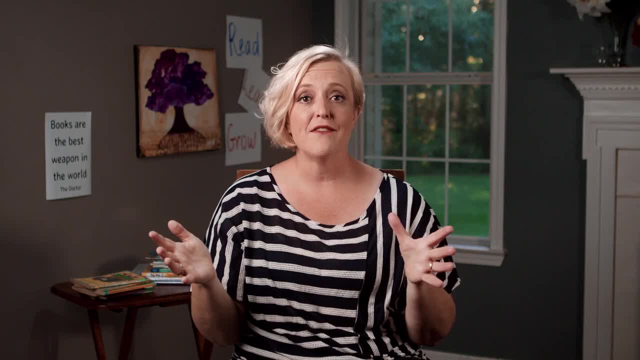 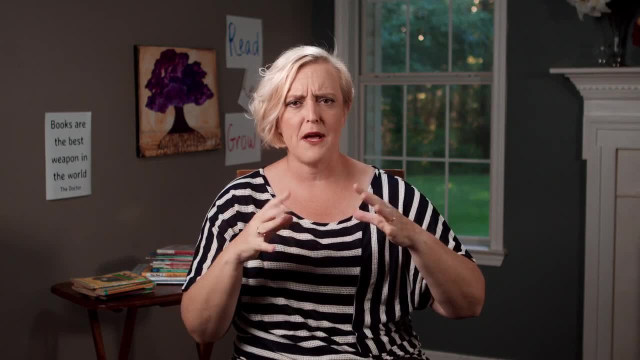 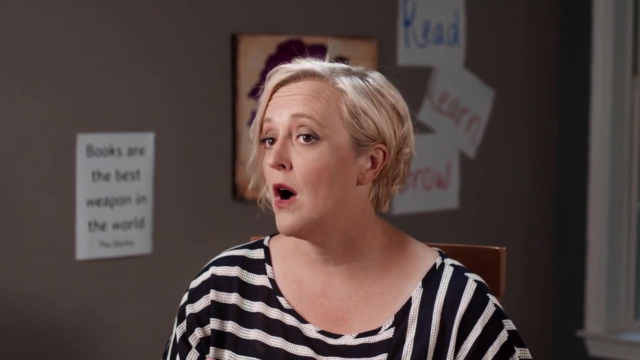 I'll never fully understand. Well, look again, I have a couple of teaching degrees and I didn't know most of the part. So the sentences you know, like the second past part, Sipples, Cousins, Twice Removed. you know, but I learned and I knew, like different parts, And so much of it was sort of in a way. 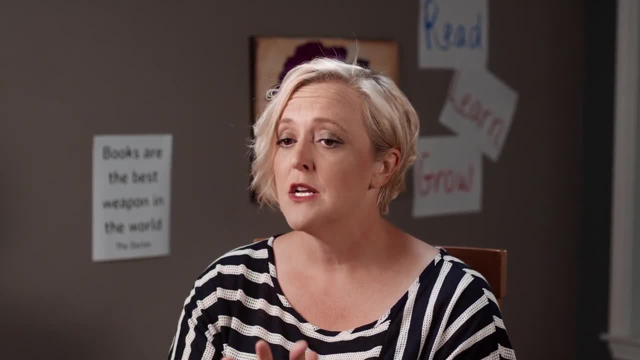 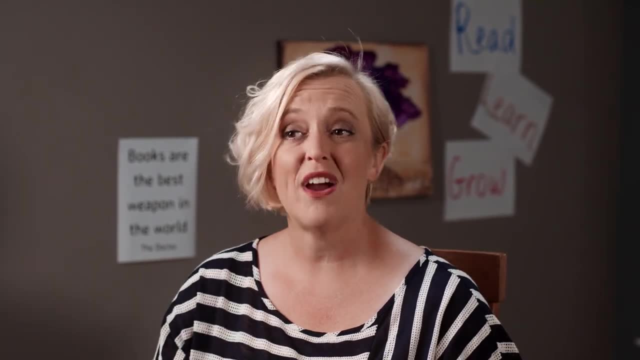 organic and how I'm bringing this across to my children as well. So some ways that we can do this: texts, emails, pen pals writing letters, cards, those things writing poetry. Don't ever forget poetry, because there's just different ways that we can express ourself. there We're going to play. 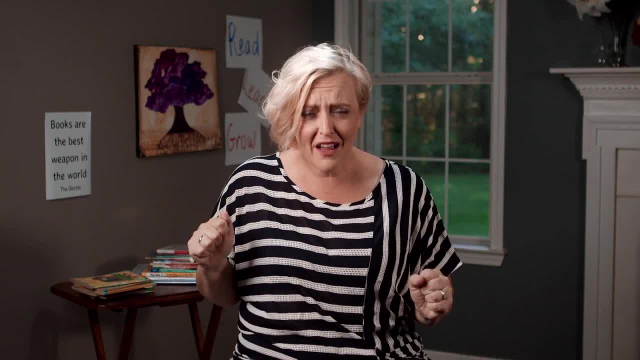 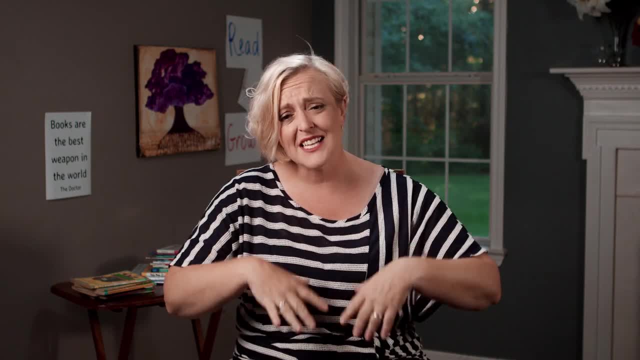 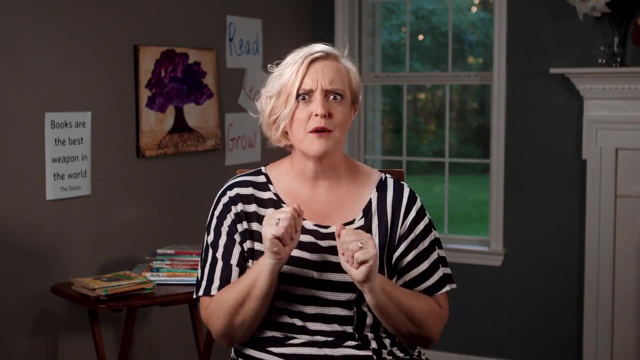 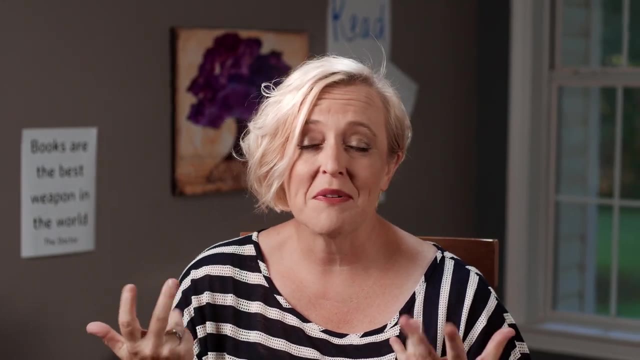 time. We're writing shopping lists, making signs, making a weekly food plan. We're writing out recipes. We're writing a story. Oh, we're writing a book. Oh, we're making a comic book. Maybe we're journaling every day or a couple of times a week. You know again so many different ways that we 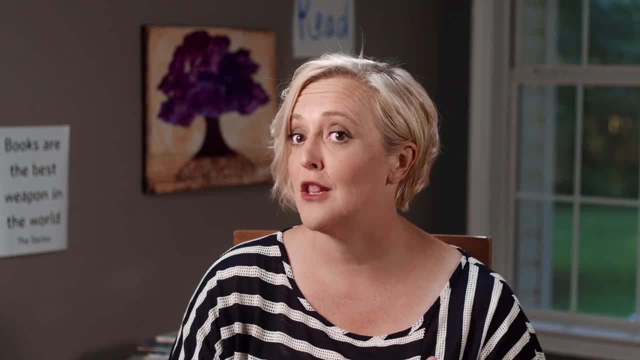 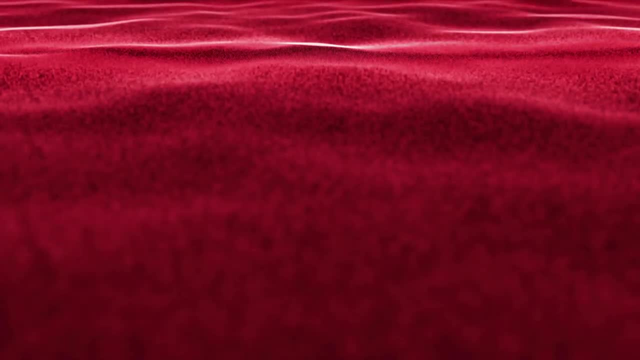 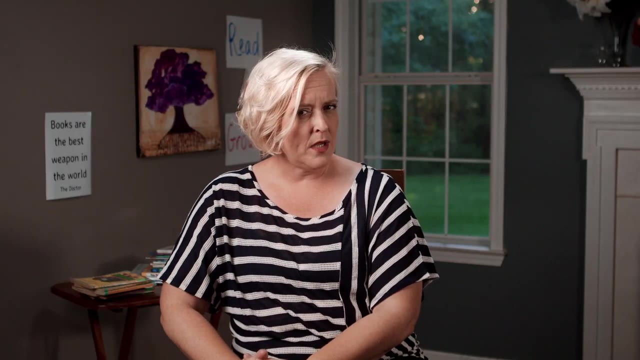 can do it. And of course, we're going to be like reading a lot, And this too, you know, we're reading our different books as we are exploring these different ideas Without formal instruction. I bet by now you're thinking: but can we? 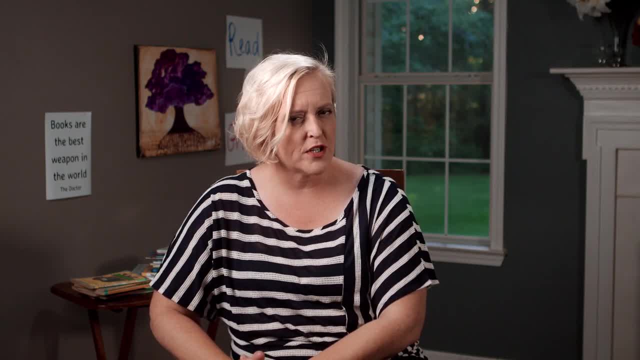 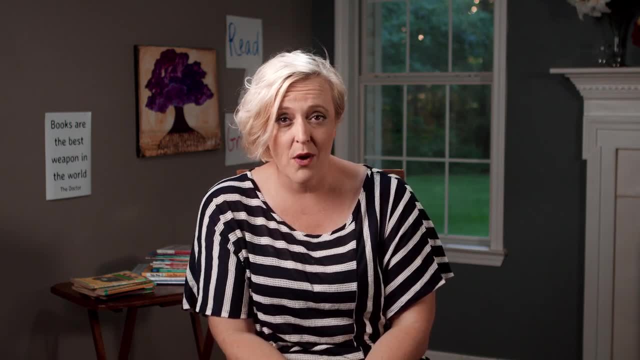 be learning. you know all of this without formal instruction. Are you really saying this, Michaela? Are you saying that we can do this? Yes, Written text is around us everywhere. Books, you know. we have this accessibility to books, you know, not just a physical form. 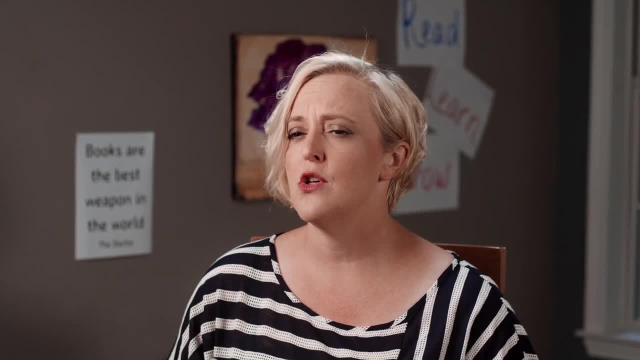 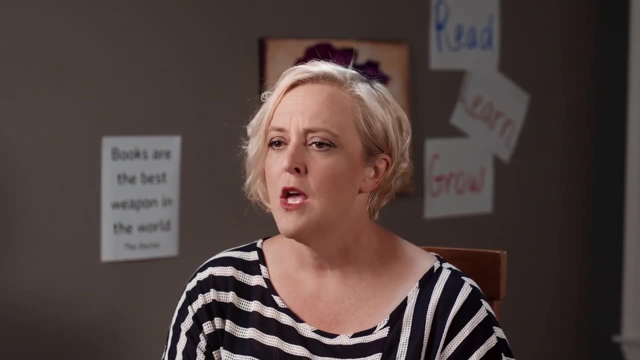 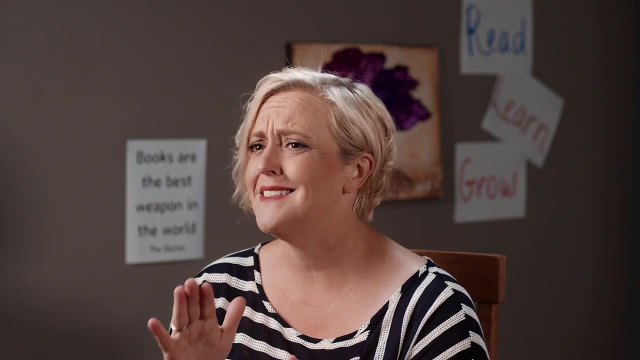 but electronically. We can learn to read and to write without that formal instruction of sitting down and following a curriculum. You know we are making sure that we are using a variety of reading material Now: our fiction, nonfiction, magazines, newspapers, websites, newsletters. 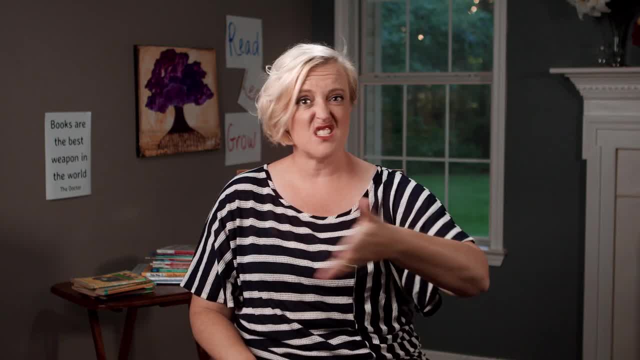 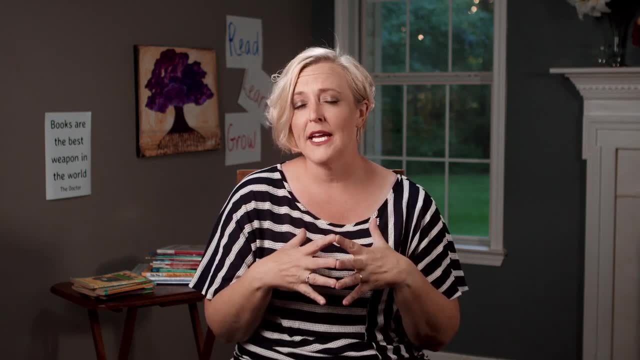 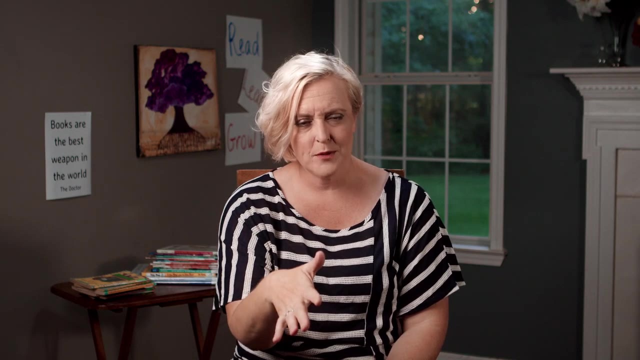 You know what? Why not go ahead and put subtitles on a show that you're watching? You know it's around us there, right? And I always say, like it's great to start with what your children are interested in, Try not to impose what you think that they should be learning, Because the number one killjoy in all 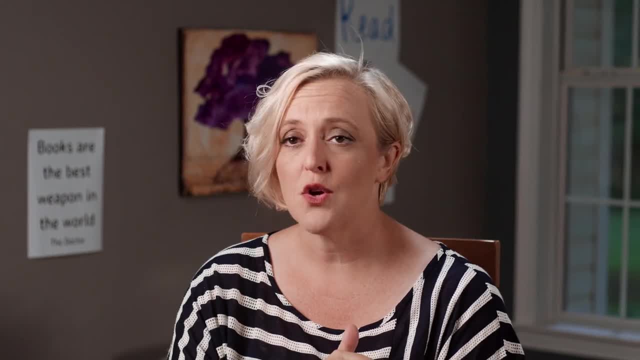 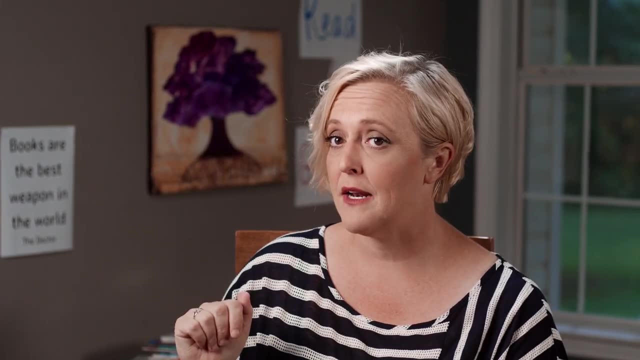 of this is having to do something you're really not enjoying. So they want to learn all about animals, and you read books about animals and you write about animals. Oh, they want to learn about another country. Then you read about that country and you write about that country. 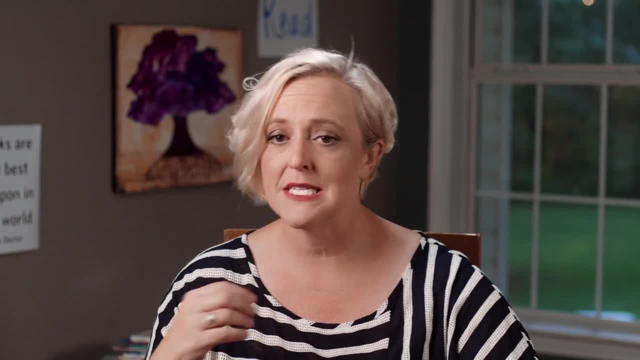 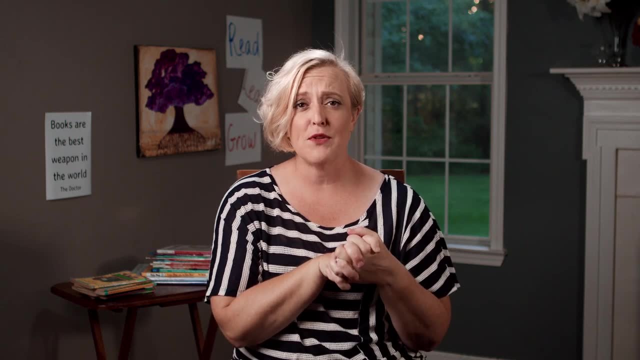 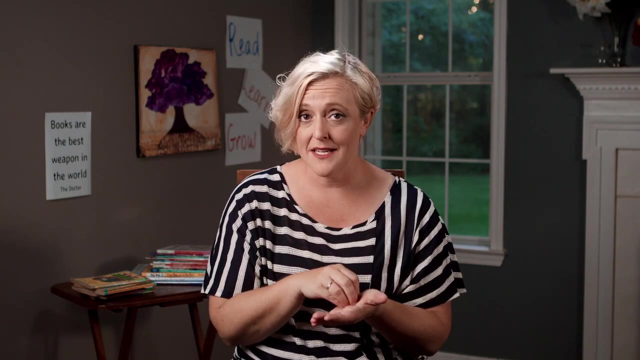 And from that you know we are seeing spelling and we're seeing all of this. You know we're introducing chapter books early. I think I started reading chapter books to my girls when they were three so that they saw how stories develop. Now also, remember you get better at writing by doing more writing. Okay, We're. 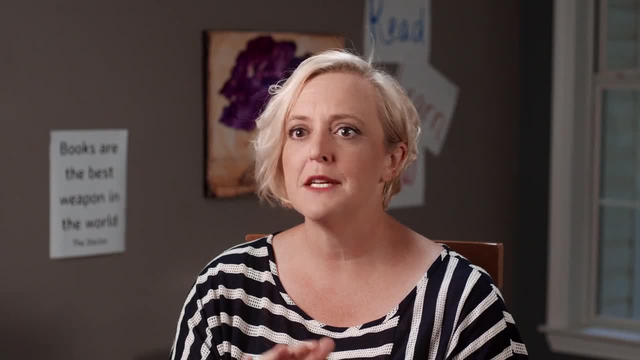 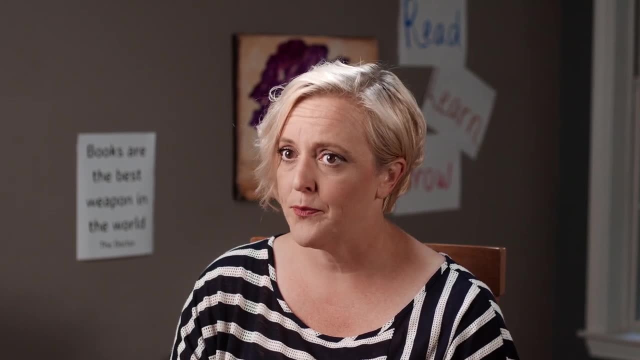 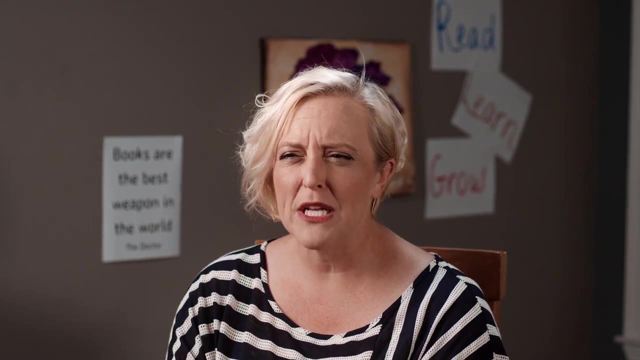 writing stories we're editing, we're going through. So writing begets writing. You know it builds up as well as reading. Good writers are good readers, Okay. So we really can't pull them apart, because as we read and we see how words are being used, from there we learn. 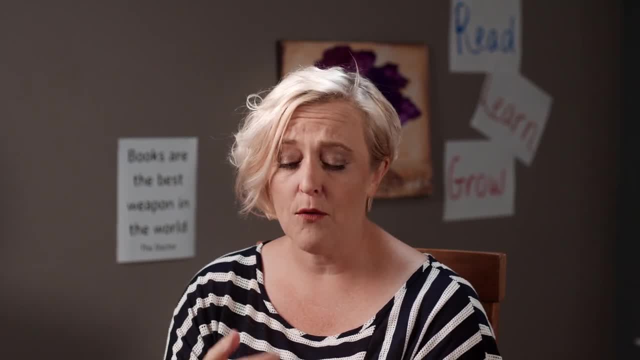 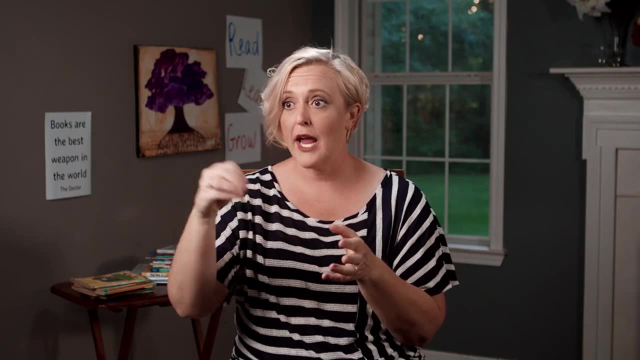 like, naturally, some of the rules that we have. We're learning about punctuation, We're learning about context and meaning and all of those different things. So write, write, write, read, read, read. Really, that's what it comes down to. But yes, you can go to the theater and 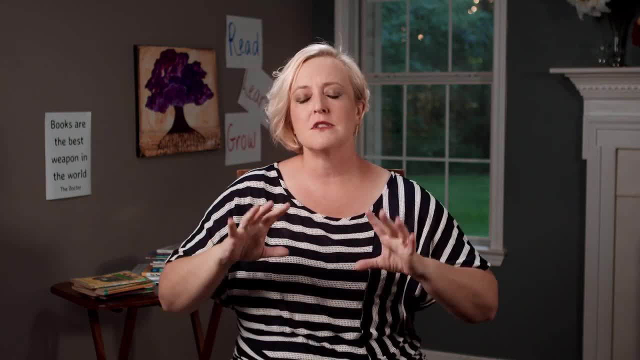 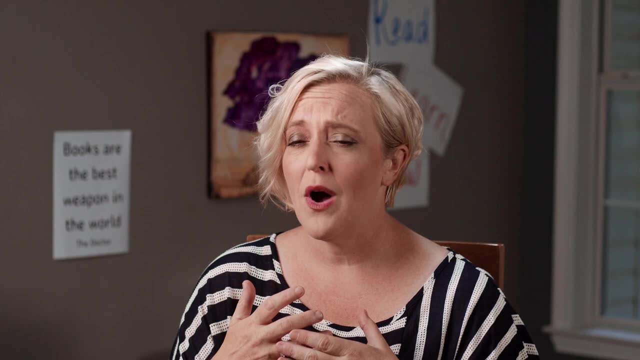 the movies and explore drama and music, because they are very valuable tools as well in exploring the object. So that's what we're learning about: punctuation, Organic learning of language arts. You know, you don't have to have phonics curriculums, You. 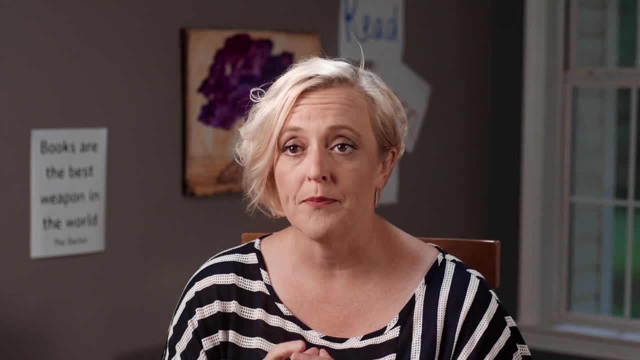 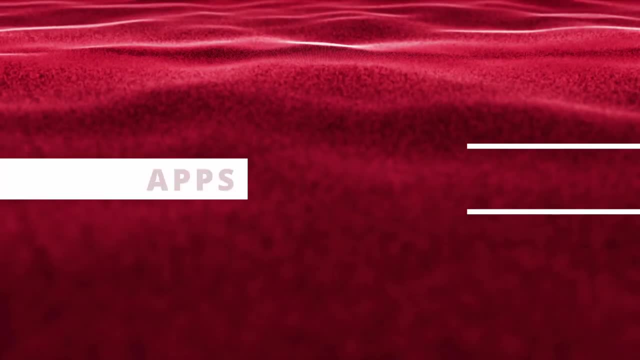 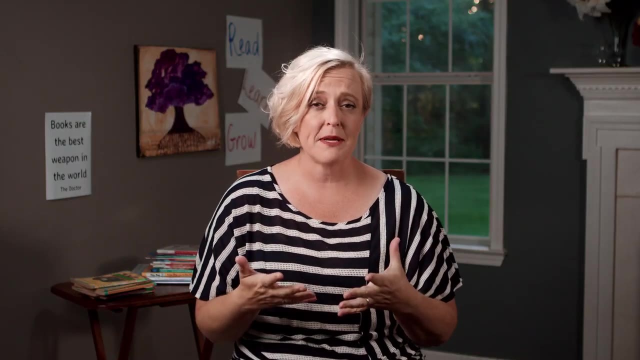 don't have to do all of this, but by reading, reading, reading and then giving opportunities to write, write, write, you are going to be able to do it. Apps for language arts: There are some great apps out there. I really do admit that, Like I love using technology, 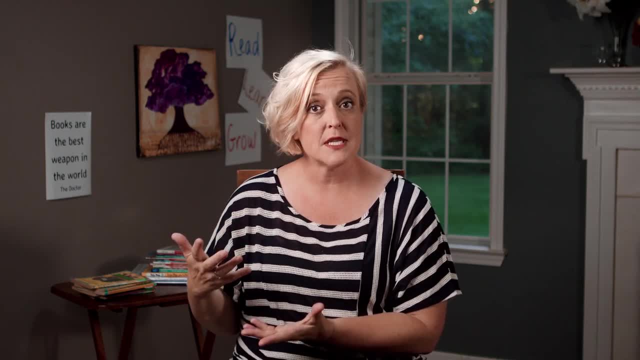 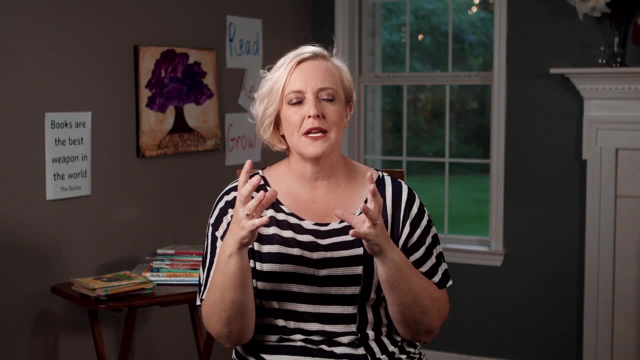 I love allowing my girls the opportunity to explore some of these apps. One that we all love is I could teach my monster to read. I get to create a monster and you teach, And I realized from that- my girls thinking it was a game- how much of learning how to build up. 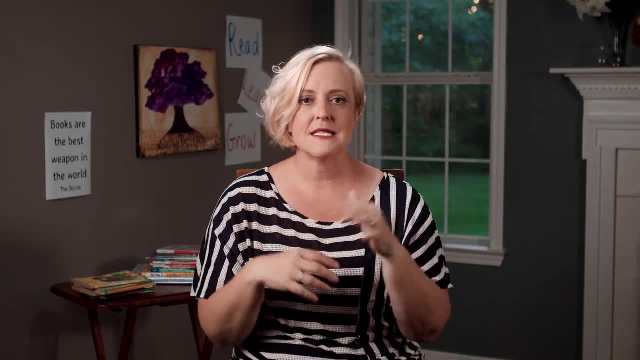 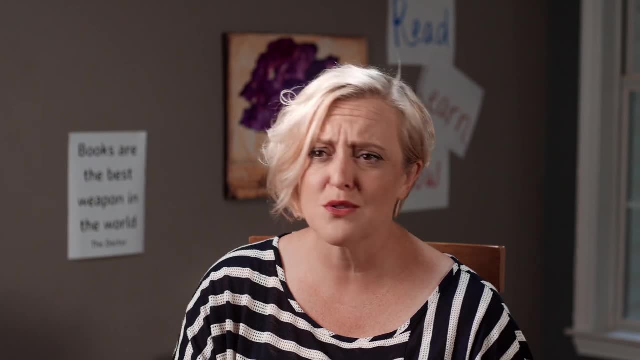 words was in it and listening for sounds: beginning sounds, middle sounds, end sounds. So that's a great app, You know, check out like different word searches and word puzzles and scrambles. They are all great, especially for spelling, you know, and you can have them easier. 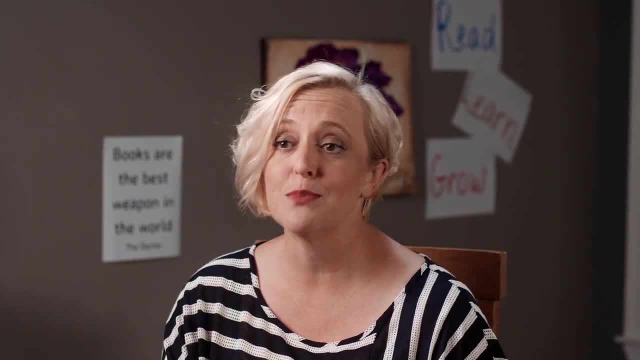 And again, it doesn't even have to be a word. It doesn't have to be a word, It doesn't have to be a. You know, you could create your own. There's books of them, And then one that I say like within. 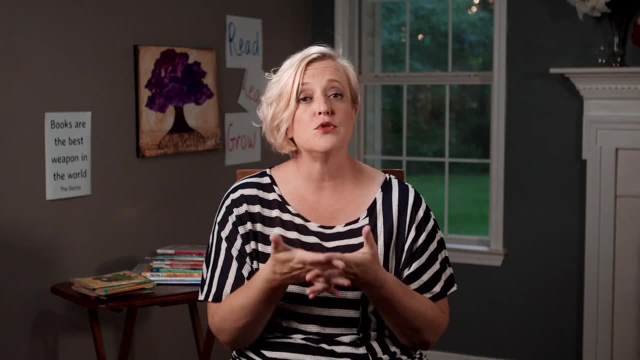 reason I don't like it as a curriculum And I know that people do use it as that And that's great. You do what works for you. But ABC mouse, you know my girls we use that as like a little. 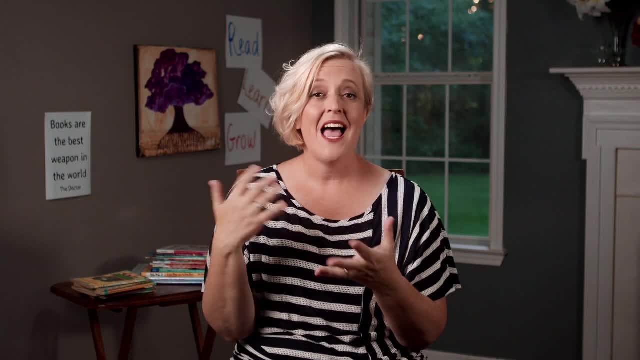 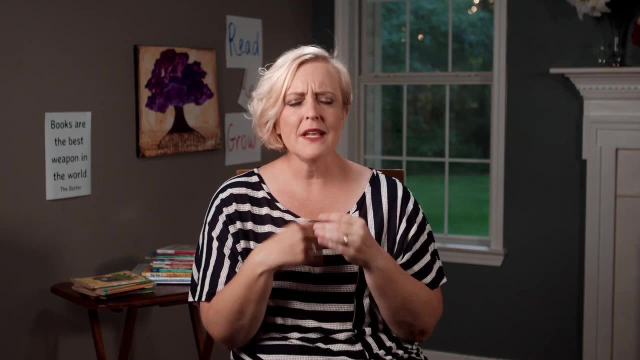 enrichment thing. you know that it's something that they can explore and you know they love the books on there and the different activities, but it's not something we do every day. It is just an enrichment. but there are some really good resources on there. 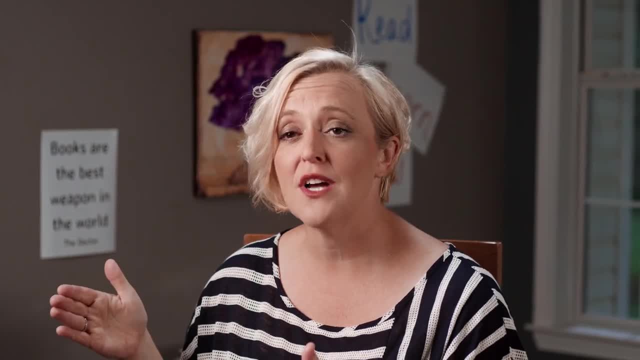 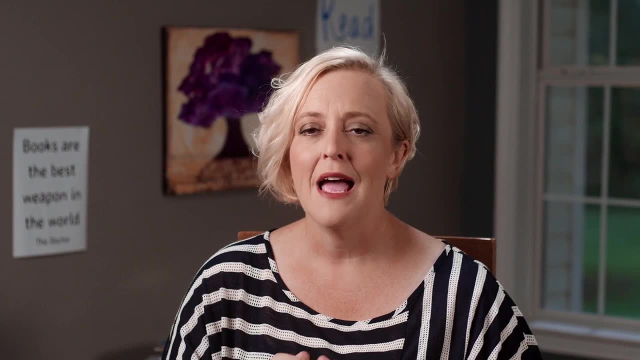 So can we unschool language arts? Yes, yes, yes. All of these we can and we can have a lot of fun with it And, like truly- and I mean that- like it is so much fun when you get to just explore. 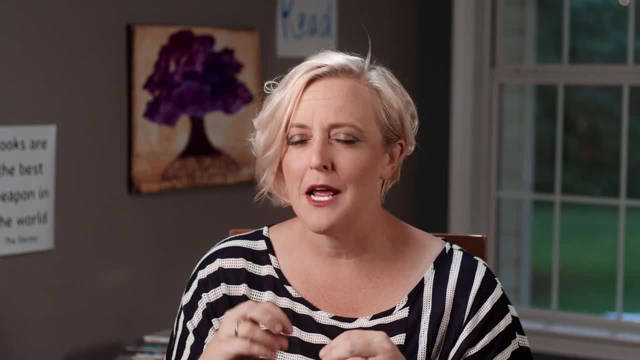 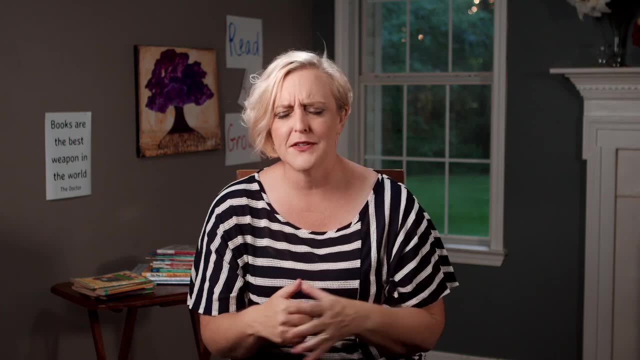 the interests that your children are interested in and finding good quality like books that you can read about it and websites, And then, like all the writing activities you can do on it, you can have so much fun that it's not bogging them down and you will see spelling improve.